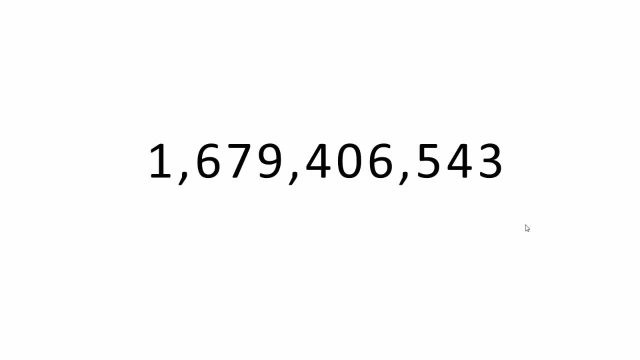 In this video we're going to go over how to read big numbers in English, and then we're going to do a listening exercise. So when looking at a number like this, a helpful tip is to remember that all commas have a name. The first comma is called thousand, the next comma is million, the next 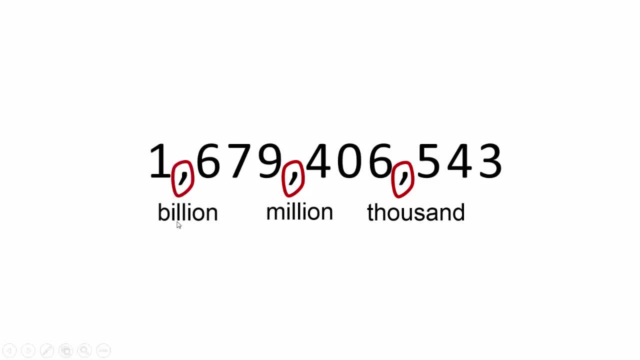 comma is billion, and there would be one more comma to the left, and that one would be trillion. Also, each column has a name, This one's one, so like one, two, three, This one's tens, ten, twenty, thirty, forty, and this one's hundreds: one hundred, two hundred, three hundred, and so on. 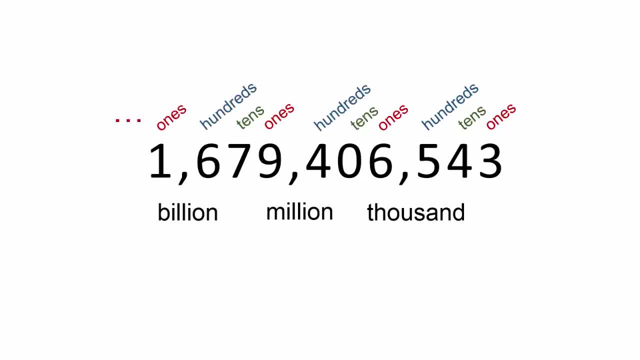 And that continues: One's tens hundreds, one's tens hundreds, and so on. So when you have a number like this, it's very easy to read: One billion six hundred seventy nine million four hundred six thousand five hundred forty three. 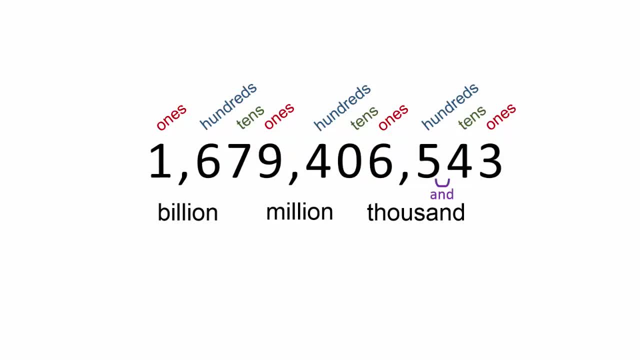 Now, if you're going to read a number like this, you're going to have to remember that all commas have a name. So when looking at a number like this, you're going to have to remember that all commas have a name. Now, quite often we also say: and between the hundreds and tens. so we would say five hundred and. 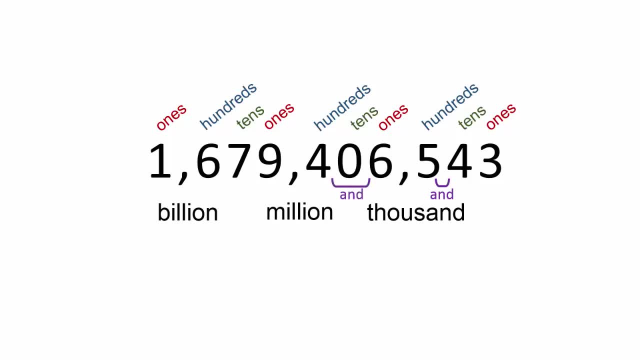 forty-three, And you also say and between hundreds and ones like four hundred and six, six hundred and seventy-nine, And we also read numbers usually in groups of threes. So if you look at the first one, let's read this again. So I would probably say one billion six hundred and seventy-nine. 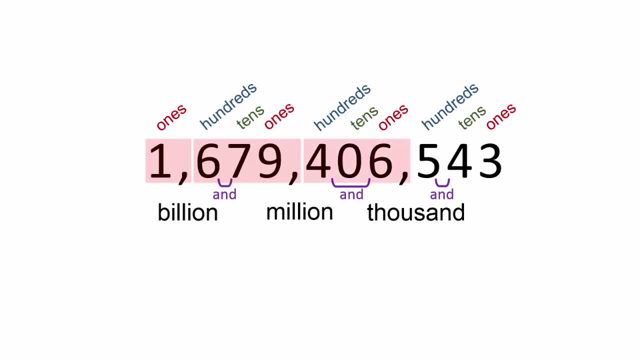 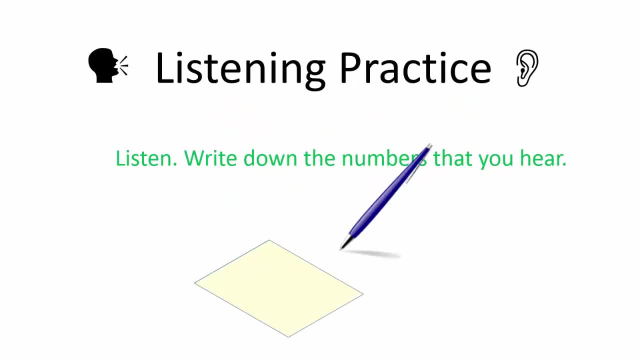 million four hundred and six thousand five hundred and forty-three. So what we're going to do is let's do some listening practice: Listen and write down the numbers that you hear. You're going to need a pen and paper for this activity. When you have your pen and paper, click on the green button to continue. So let's start. 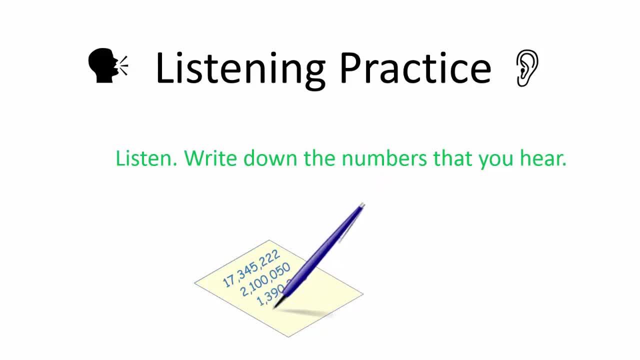 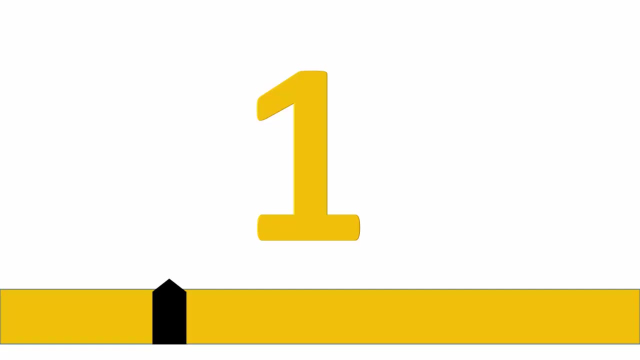 I'm going to read out five numbers. I'm going to read each number twice. As you listen, write down the numbers on your piece of paper, and then I'll show you your answers after. So here we go. Let's go. One million six hundred and seventy-eight thousand nine hundred and fifty-seven Again.